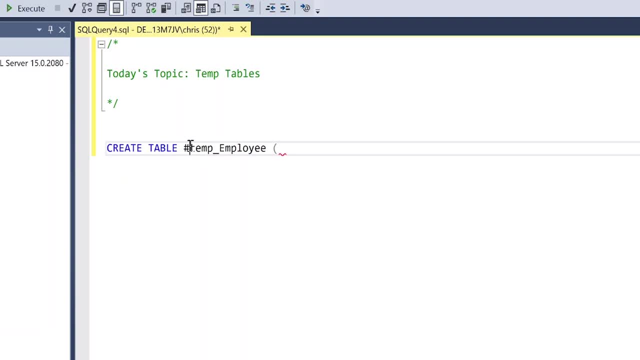 the only difference between a regular table and a temp table is this, right here, at the very beginning: this, this pound sign. So, uh, let's just start by doing employee ID, We'll make that an integer, We'll do job title and we'll make that a varchar 100.. And then 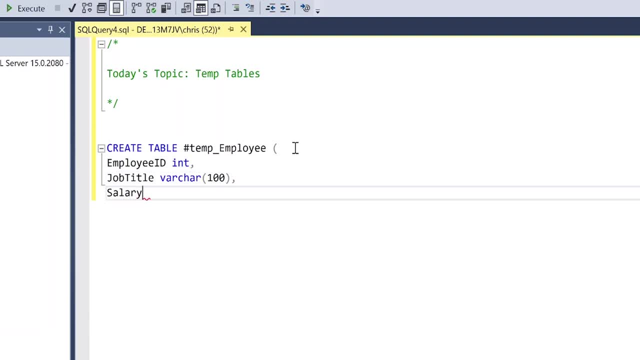 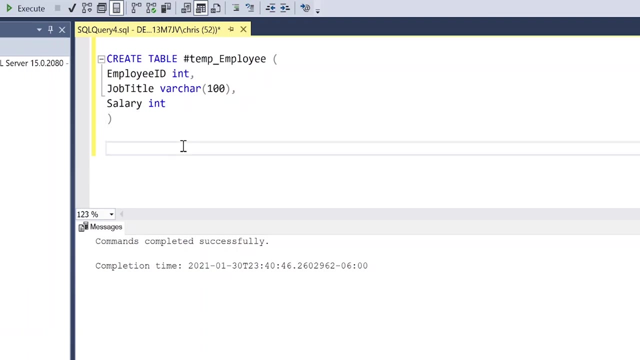 we'll do salary and let's make that an integer. And so now we have our temp table. Uh, let's go ahead and create it. So now we have our temp table created and so we can look at it really quick. So let's select everything from and we'll do temp employee. So let's take 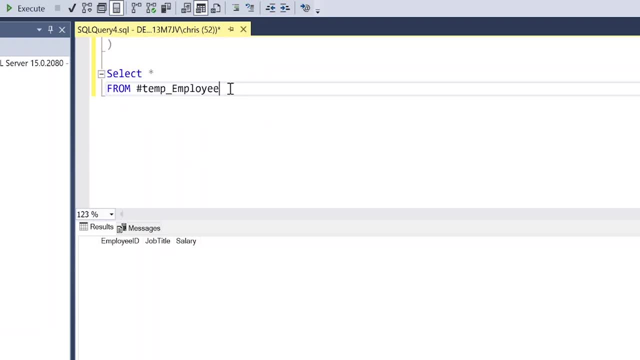 a look, It's completely empty, Um, and we can insert data very much the same way we'd insert data into a regular table. So let's start doing that, Let's do insert into and we'll do temp employee and we'll do values, And let's just do something really quick. So I'm going to 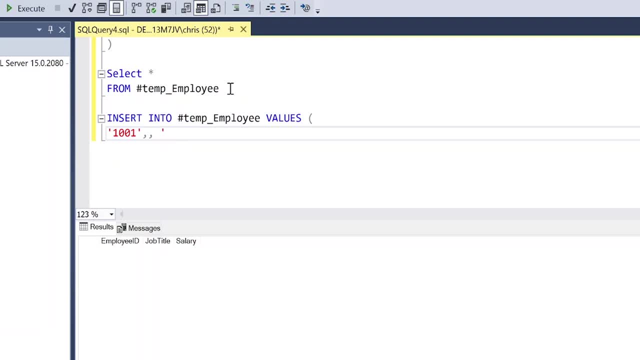 get to a little bit more interesting stuff in a second Oops. So we'll make this pretty quick. So we're going to go ahead and do this person HR- uh, their job title- and then for salary we'll give them 45,000 and close it off. So let's run this and let's select everything. 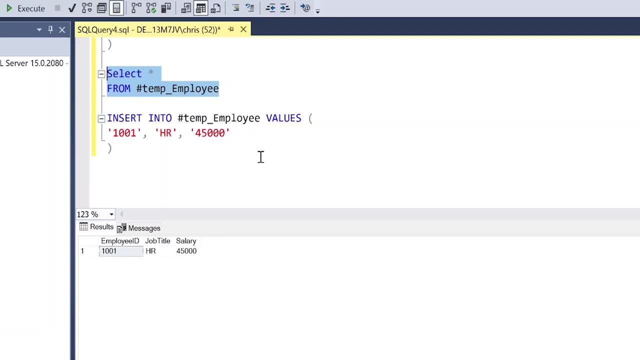 again and see what's in there- Perfect. So we were able to insert data into this temp table And again we ha. we don't have to create this every single time, we um, or we don't have to run this every single time. we need to hit off of it Like we did a CTE, If you. 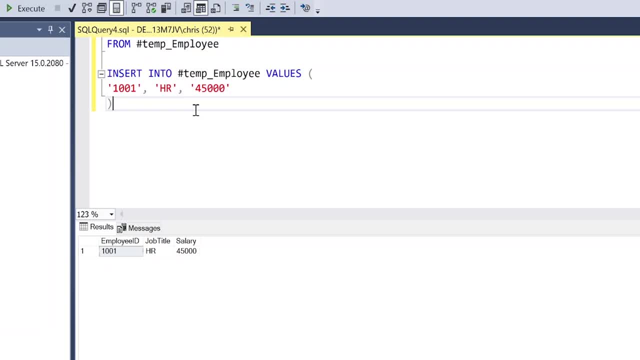 watch my previous video, uh, and this one. we can just run it and it sits there And so, um again, it feels very much like a real table, and I'm going to get to a little bit of the nuances of of the in the differences between a regular table and a temp table in. 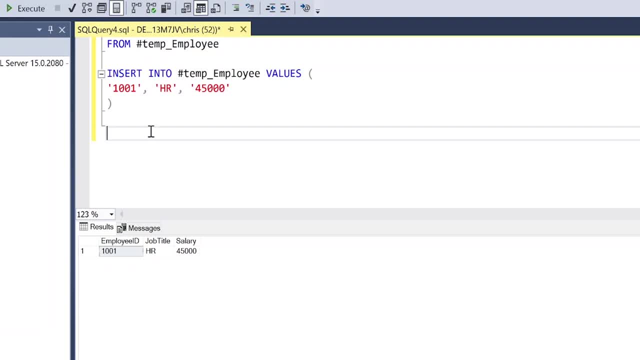 a second, but let's really quickly. Um, we want more data in there. You don't have to just um, do it value by value. We can also just do um, uh, where we select all of the data from a specific table and insert that into a temp table, And that is really quickly. 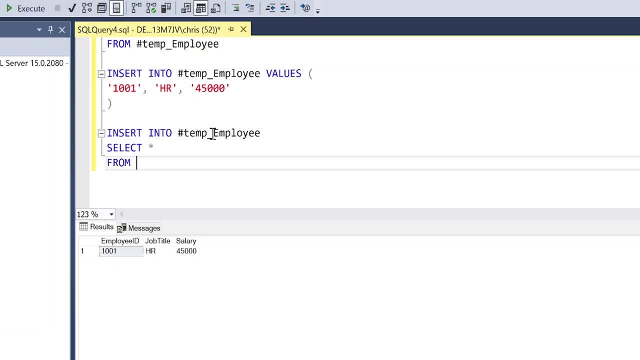 you know how I do it: Most of the time, most of the time, I'm not inserting values. Um, I am, you know, taking a large table and taking a subset of that and then sticking it into a temp table. So let's look at this really quick and run that. So now we took all of 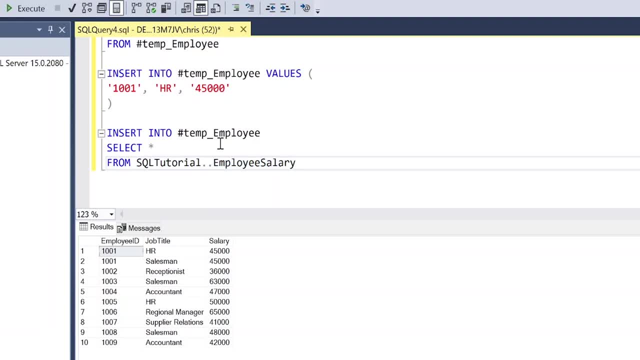 the data from employee salary and then we just stuck it into this table, And really quickly. this is one of the big uses of a temp table We had. let's say, for example, that this employee salary table had a billion rows, or or or just an extremely large number. 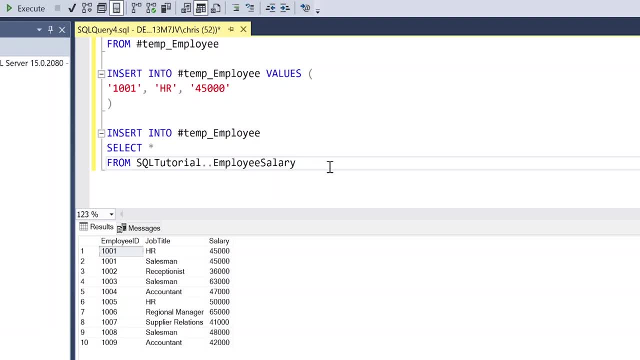 And we were trying to, uh, you know, hit a somewhat complex query off of it, where we're using joins and we're using, uh, maybe some window functions or different things. Um, you know, it would take a very long time to hit off of this, but what we can do is: 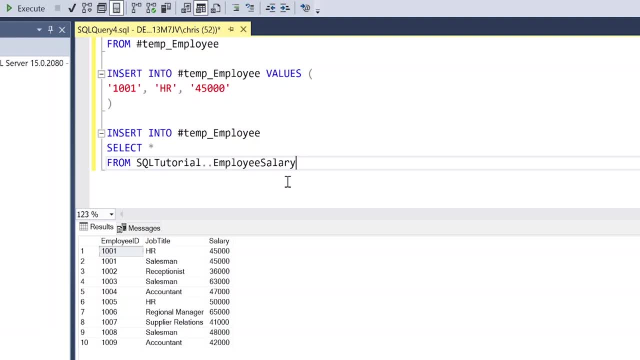 we could insert that data into this temp table and then we can hit off the temp table and it already has that sub, uh, that subsection of data that we're wanting to use for all of our later queries. So, really quickly, that's kind of um, kind of a use case for that. 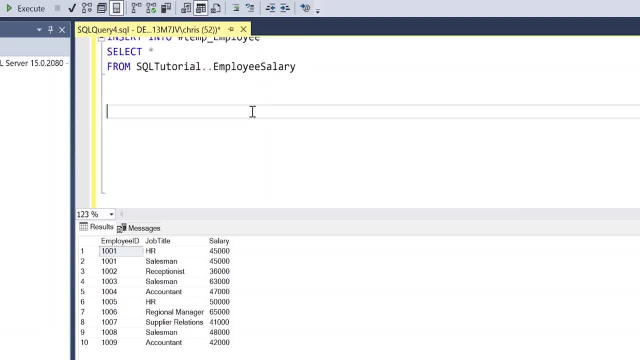 So let's go down here. We're going to kind of create another one, and this one's going to be a little bit more advanced and a little bit of how I would use it. I would actually use a temp table. above was just kind of showing the basic syntax, how. 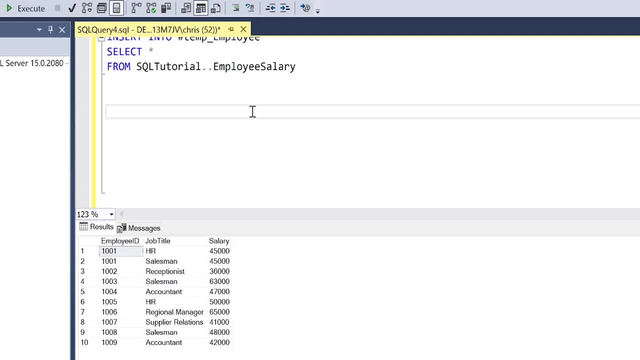 you kind of put data into it. you know kind of how it's used. Now I'm going to show you kind of how I would actually use it. So let's do create table. Uh, let's do temp- Oops, Great table. Uh, let's do temp- uh, employee two. and then let's do open parenthesis and 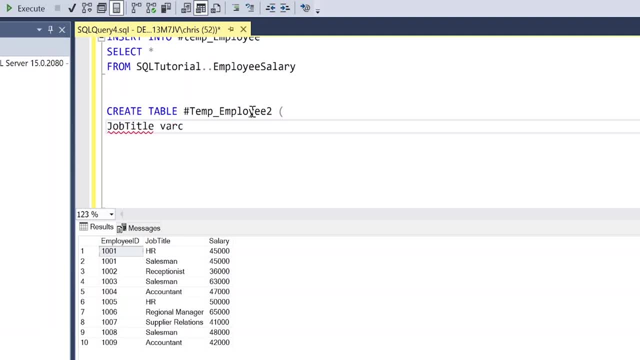 we'll do job title. We'll make that a bar char 50, and then we can do employees per job. We'll make that an integer. Now we need average age. make that an integer, and the very last one will be average salary. I'll make that an integer as well, And let's run this Oops. So we have. 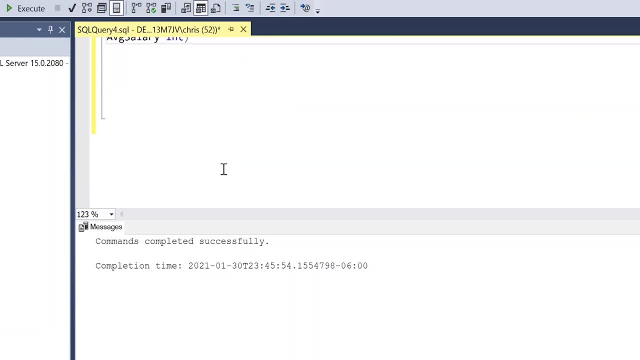 our second table. Now we want to insert data into this one, So we're going to just going to do insert into and we'll do temp employee two. And for this one I'm going to take a query that we used in a previous video And so I'm just going to copy and paste that to save time. 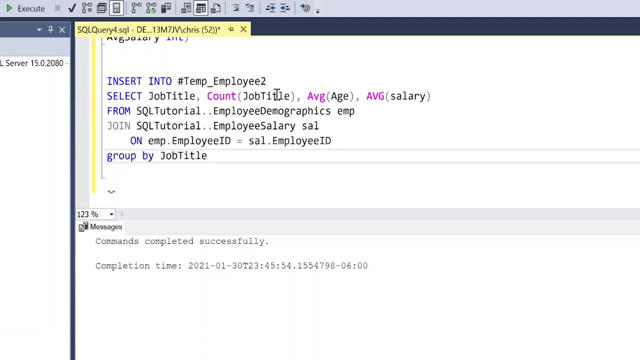 Uh, and then we'll keep on moving from there. All right, So I'm just going to paste that in. We will run this and really all it's doing is from this, from these tables, it's taking the job title. We're getting an account on the job title: average age, average salary. 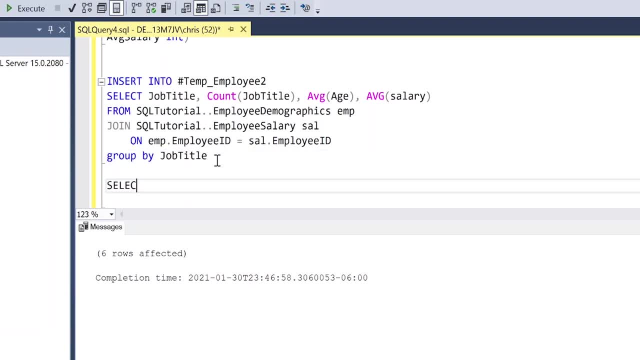 and that is it. Um, so let's see if that worked, which it looks like it did. but you know, let's actually take a look at the data, And so now we have this subsection of data from this join above, And what this is going to do is, whenever we want to run this, we don't 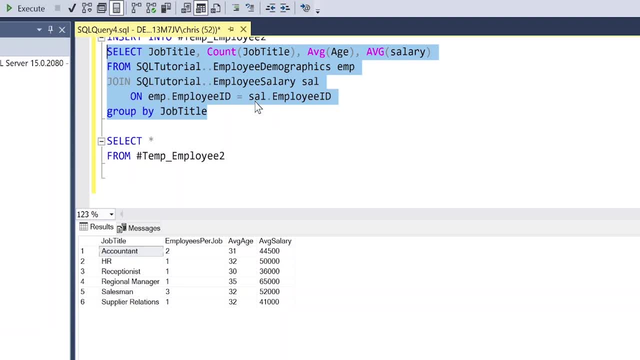 have to run it on these two tables- Speaker 1- And create the join and then do the calculations, which takes time. What it's going to do is it's going to take this, these exact values, and places into this temporary table And, if we want to run further calculations on 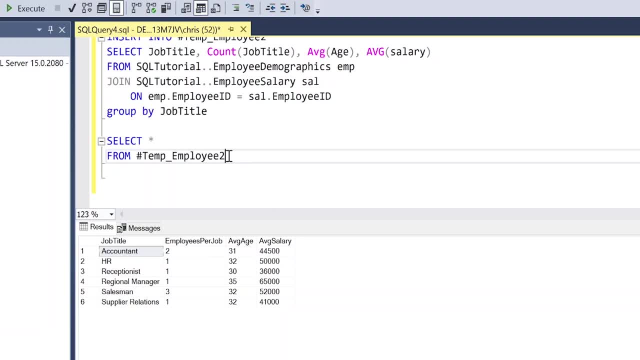 these values. we can easily do that in a fraction of the time instead of having to run this every single time, which will take up so much uh uh processing power, And it will reduce your runtime dramatically when you're placing this data in this temp table and hitting off. 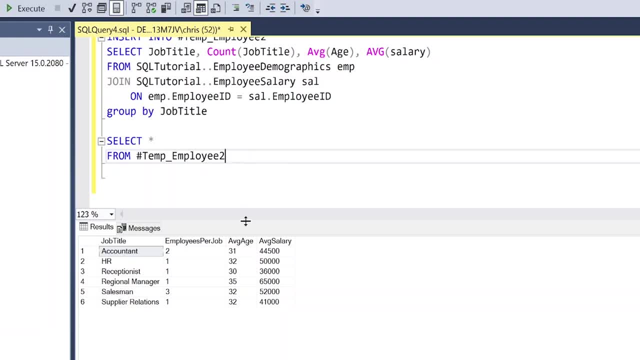 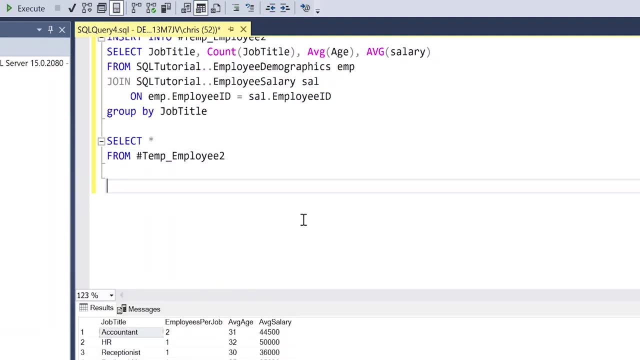 of that. Speaker 2: So all these joins and everything above. uh, a lot of times these temp tables are used in store procedures. Now, if you haven't learned about store procedures or used stored procedures at all, you know that's okay. I still want. 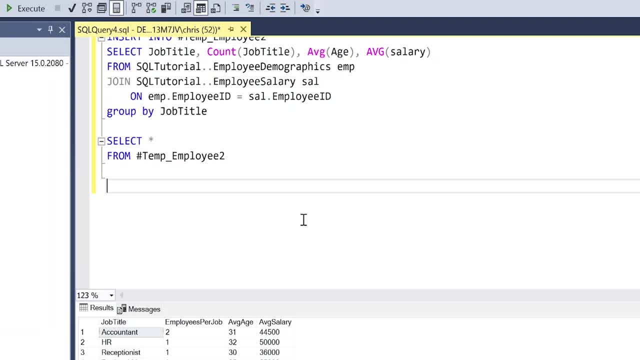 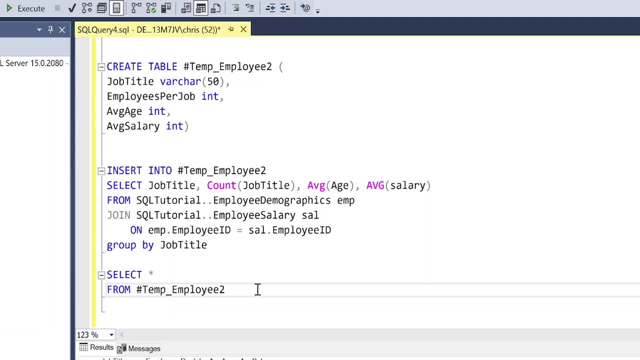 to show you something that might be useful. Um, although this is used a ton in store procedures. So, for example, let's say we have a store procedure set up, we run the store procedure and we get an output. and you know, we forever reason want to run it again. And when we run, 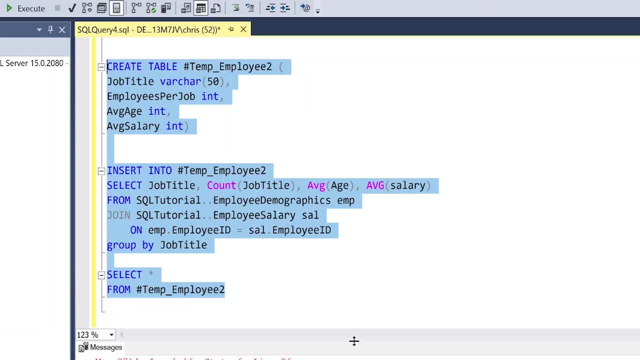 it again. uh, we get this error. Speaker 2: And you know, this temp table lives somewhere, It it. it doesn't live in an actual, in the actual database, uh, but it lives somewhere. And so when we run it again, we get an error because there's already a temp table created. 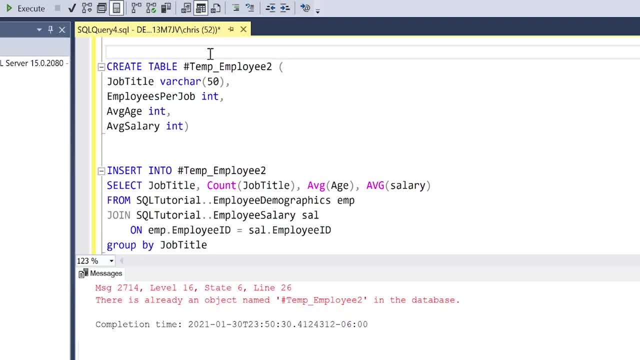 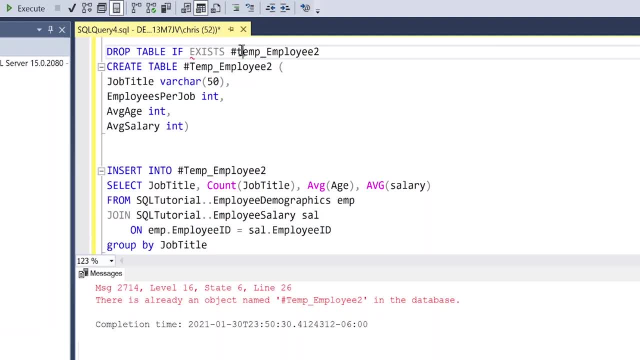 Speaker 2. So let's do temp employee to just like that. Now, what this is going to do is, when you're running that store procedure over and over and over again, you're getting an error or whatever. for whatever reason, you need to run it multiple times every time. 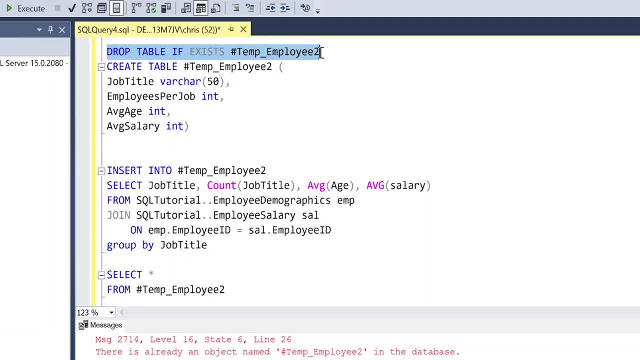 that you run it, it's going to encounter this, And so, if that already exists, it is going to delete that table and then allow you to create it again, And this is just a really good thing to do. So now, if you see down below, I can run this time and time and time again. 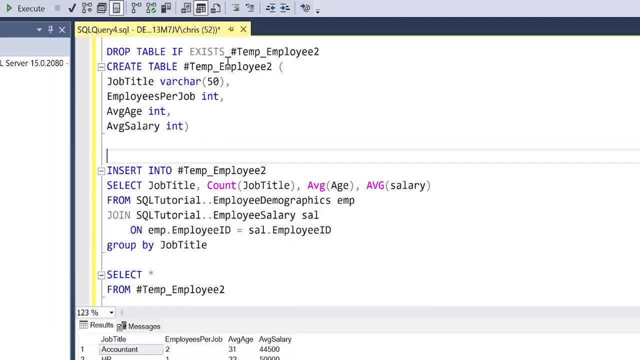 and it is going to work every single time because it is checking to see if that exists, And if it does, it deletes it, and then I can create again, And so that is just a helpful tip. If you're going to try to use this, I highly recommend adding that to your query. 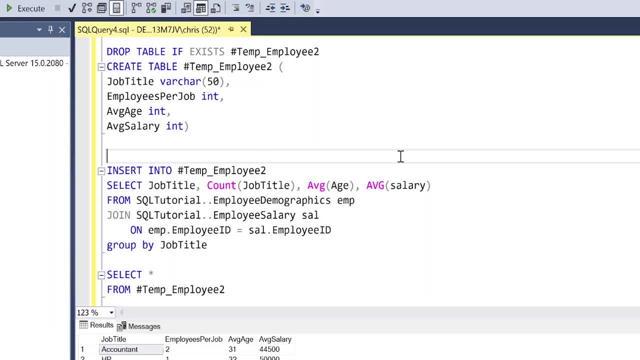 just to make sure things run smoothly. I know there is a lot more that can go into temp tables, a lot more of the technical aspects of the DBA stuff, Obviously. I just want to teach you how to use it and what you might use it for and how.